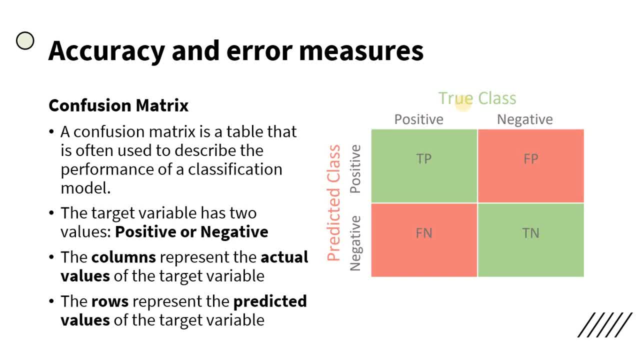 Here true class means the actual value And the predicted class means what the model predicts: Yes, so let's understand each of the term in detail. So here the first term is the true positive. Here TP means true positive. Here let's understand with one example. suppose I am suffering with some disease and I visit to the doctor and after checking doctor says that yes, you are suffering with jaundice. 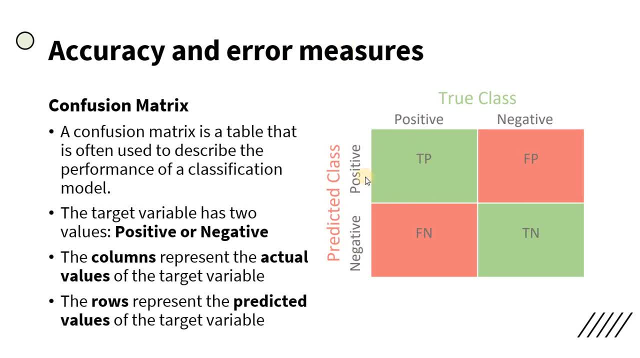 So here doctor provides: is it's a positive review. so here this is a P means positive. So predicted class means doctor predicts that it may possible that you are suffering with the jaundice. so that is why here P means positive. Here first is a T means true. So doctor provided his review that you are suffering with the jaundice. 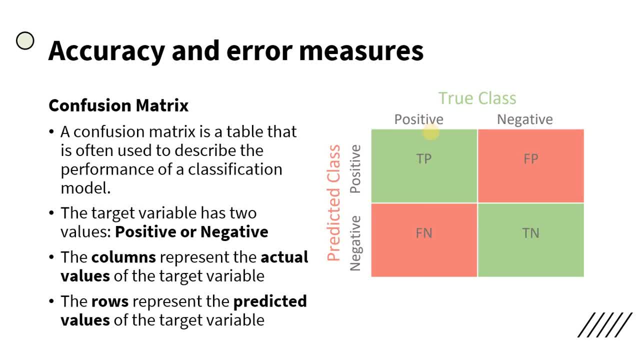 After getting the reports, it is possible that you are suffering with the jaundice. This also shows that you are suffering with the jaundice. Your jaundice is a positive. So here, both prediction of the doctor and the values in the report, both are true. 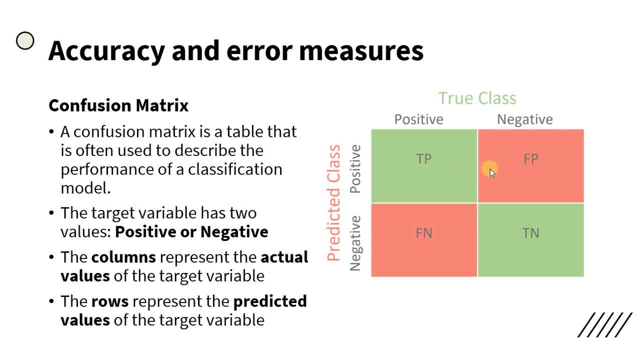 So that is why it becomes true. positive Same as false. positive means doctor says that you are suffering with jaundice, So doctor's review is positive, but report says it's a negative. It means the decision of doctor, The doctor, is negative, false. That is why we are writing here as a false positive. 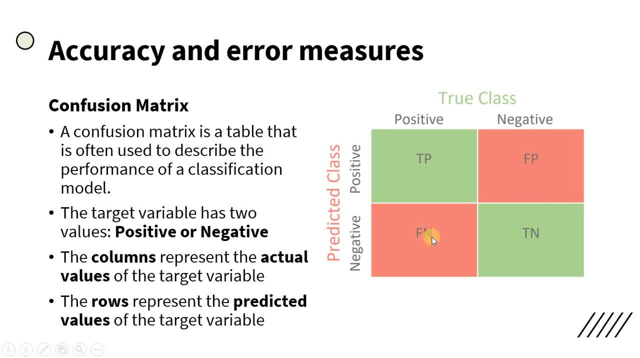 Here. third one is a FN means false. negative Means doctor says you are not suffering with any disease. So the doctor decision is negative but report says positive. So here the decision of doctor is not true. That is why false negative. and the fourth one is true. negative means doctor says you are not suffering with the jaundice. 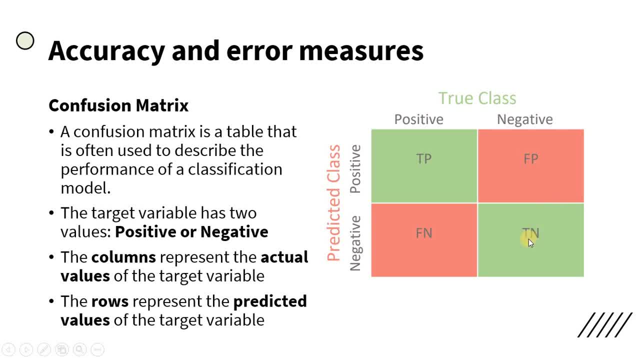 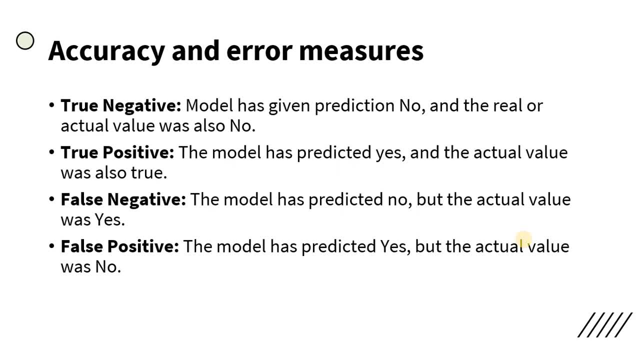 And also report says you are not suffering with the jaundice, which will become true. So that is why it becomes true negative. I hope this is clear to you. The true negative means modulus has given prediction No and real actual value was also no. 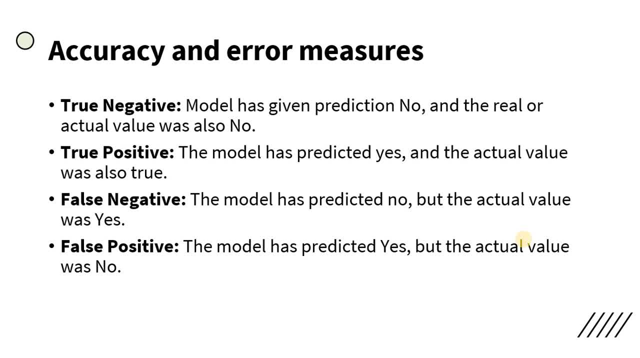 That's a true negative. Second is a true positive: The modulus has predicted Yes And the actual value was also true. Now, third one is false Negeative Means: modulus has predicted No, but the actual value was yes. and the last one is false positive means: the model has. 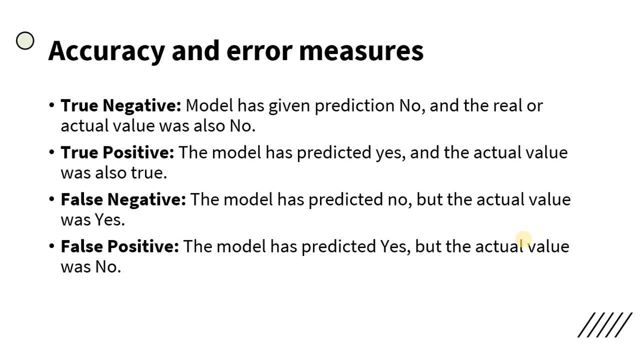 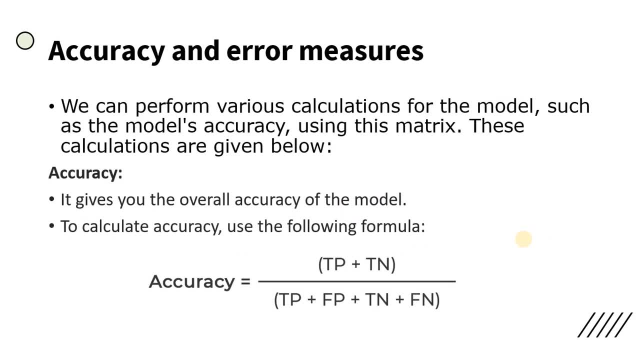 predicted yes, but the actual value was no. So that are the main parameters of the confusion matrix. Now, based on this confusion matrix, we can measure the different accuracy measures. So the first one is accuracy, so it gives you the overall accuracy of the model when we 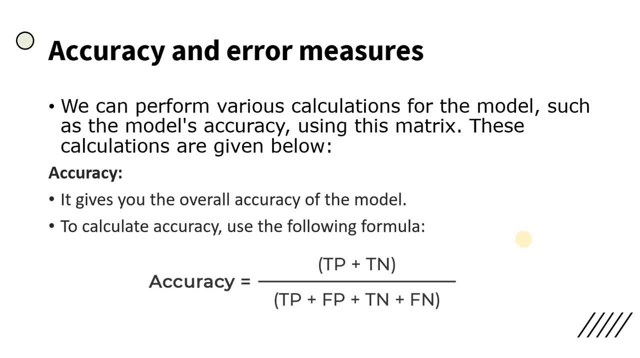 are talking about any classification algorithm at that time. mostly we are using the accuracy as a measure that how effective our model is. So for that we are using the accuracy, and the formula for accuracy is: true, positive plus true, negative divided by total means: true, positive plus false, positive plus true. 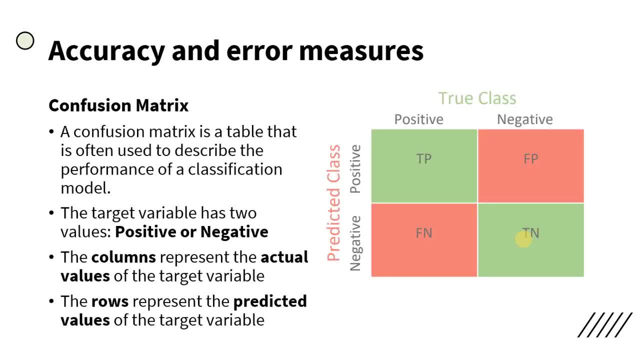 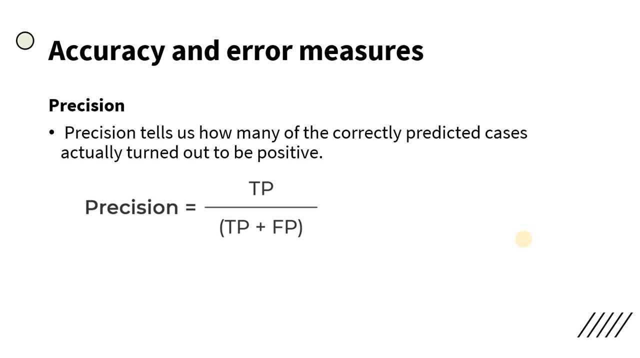 negative plus false negative, and all that value we can get from this confusion matrix. So these are the derived values, These are the derived measures from confusion matrix. Next is a precision. Precision tells us how many of the correctly predicted cases actually turn out to be positive. 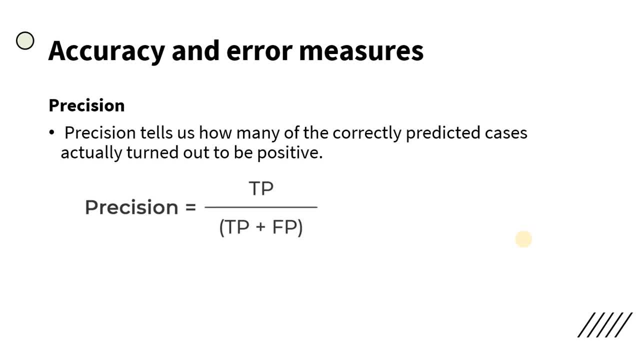 Yes, if from 100 samples the model says 80 is a positive. so we need to check that if all that 80s are correctly predicted, in the correct class or not. so that is from that we can define, from precision, Precision. and the formula is: true positive divided by true positive plus false positive. 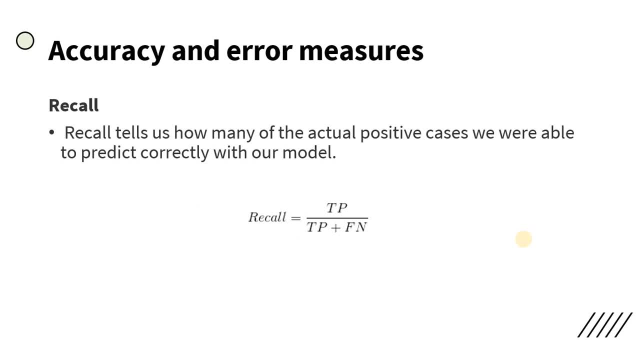 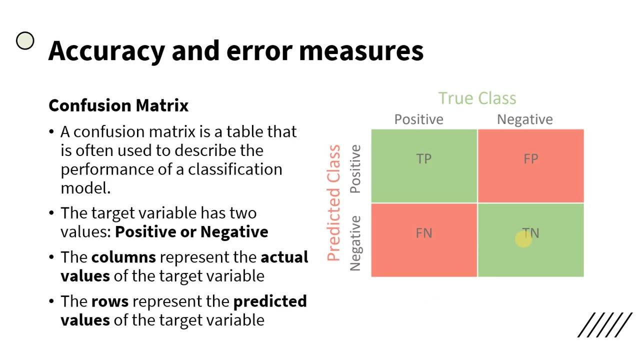 Next is a recall. So recall tells us how many of the actual positive cases will be able to predict correctly with our model and the formula is true positive divided by true positive plus false negative. So these are the main measures we can derive from the confusion matrix and this is a measures 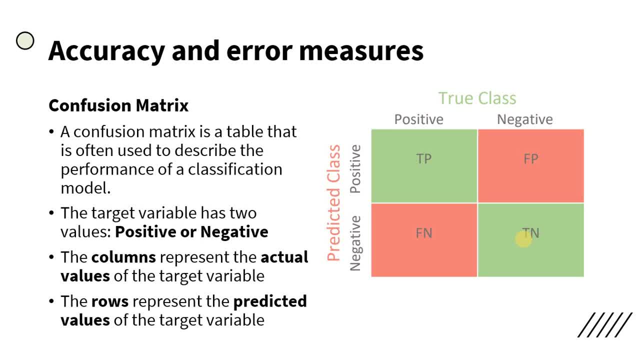 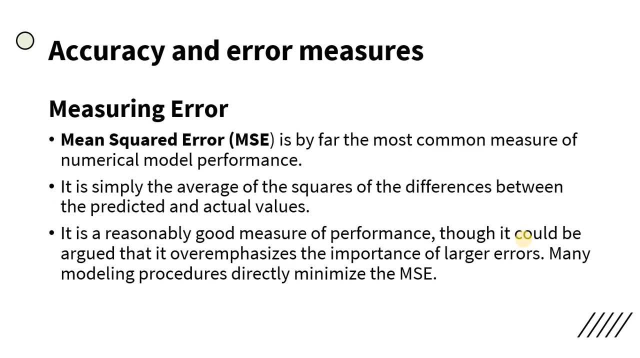 with that we can calculate or we can get the Effectiveness of our model. next one is a error measures. as well as accuracy, we need to find the errors also, that in which samples, errors are occurred, so that we can measure using some different measures of errors. and the first one is a mean square error, so mean square. 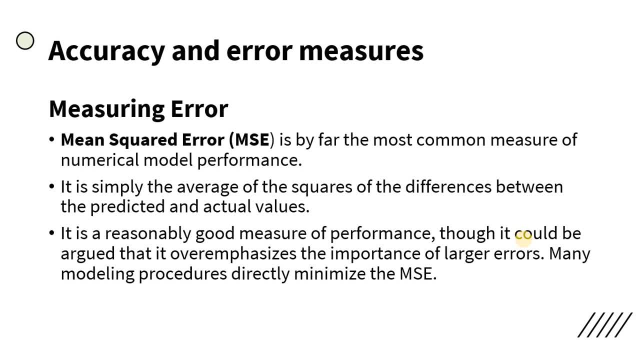 error is by far the most common measures of the numerical model performance. it is simply the average of squares Of the difference between predicted value and the actual values. it is a reasonable, good measure for performance. through it could be argued that it over emphasized the importance of large errors. many modeling procedures directly minimize the MSA, so this is the most important. 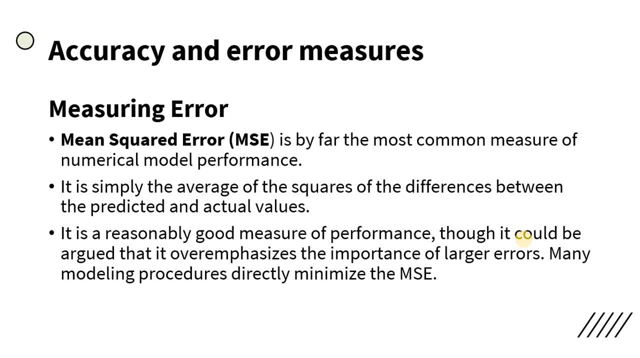 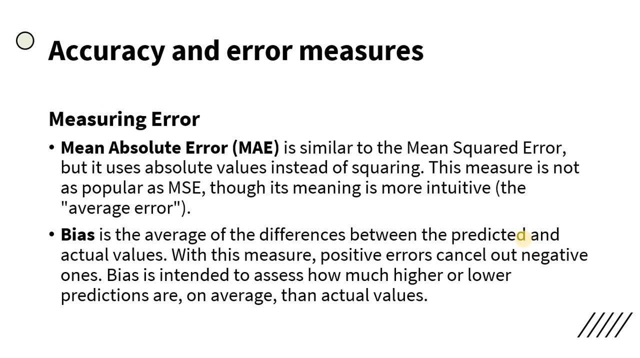 measure that is used to find out the errors, and it is simply by calculating the average of squares Of Errors between predicted and the actual values. next error is a mean absolute error. mean absolute error is a similar to the mean square error, but here we are not taking the squaring. yes, 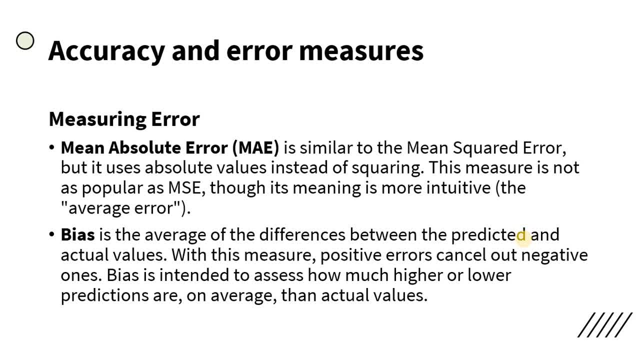 but we are using the absolute value instead of squaring. this measure is not as popular as MSA through its meaning is more intuitive, so this is not mostly used, but mostly for errors. we are using the Mean square error. Mean square error next is a bias. so bias is the average of the difference between the 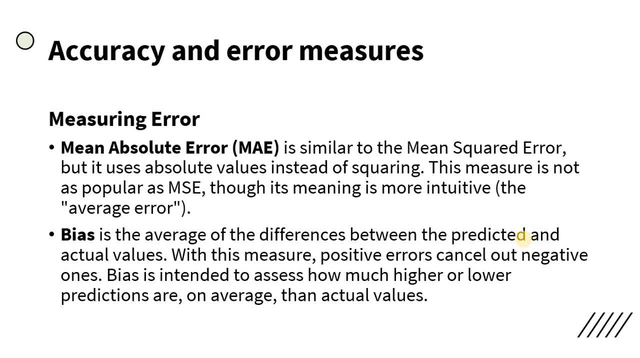 predicted and the actual values. with this measure, positive errors cancel out the negative ones. bias is intended to access how much higher or lower predictions are, or on average, than the actual value. so here we can calculate the bias also. we are providing bias value to the model, also to improve the efficiency of the model. 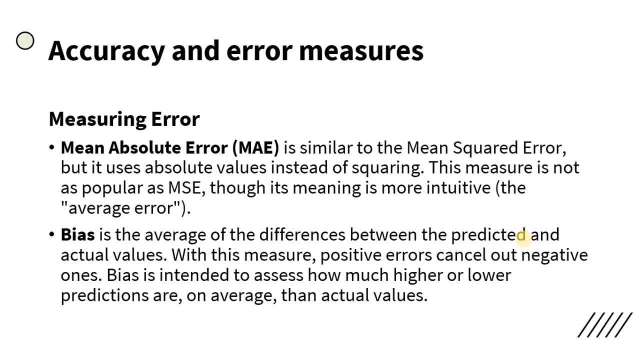 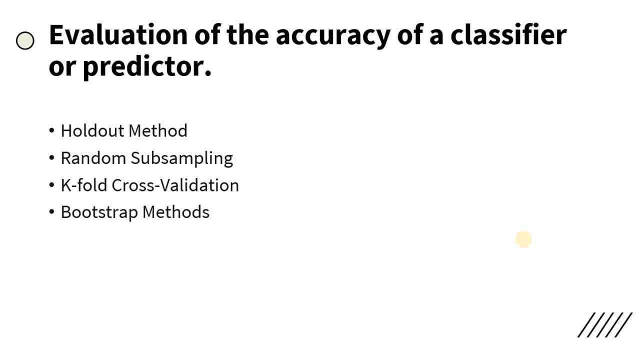 So these are the accuracy and error measures of any classification algorithms. now the next one is evolution of the accuracy of classifier, the predictor. so when we are building any classification model and then we are calculating the accuracy of the model, but by only one method, by only taking that one portion of databases, we cannot get the correct output. 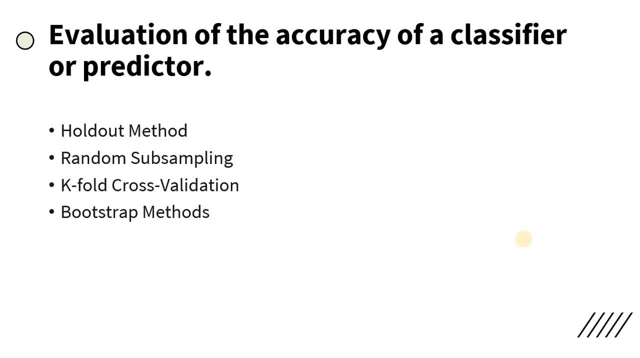 yes, So for that there are multiple Outputs. Accuracy evaluation measures are there? accuracy evaluation methods are holdout methods, random sampling, k-fold, cross validation and bootstrap methods. so by following any of this method we can get the more accurate results. so for that we are using this method, the first one. 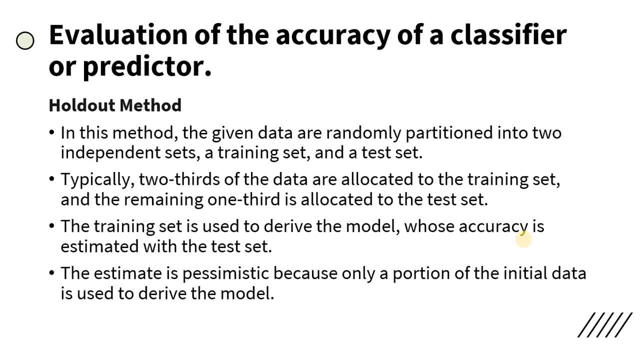 is a holdout method. so in this method the given data is randomly divided into two independent sets. Here we need to understand one thing: that for any types of classification algorithm we are using two data set. first is a training data set and second is a test data set in. 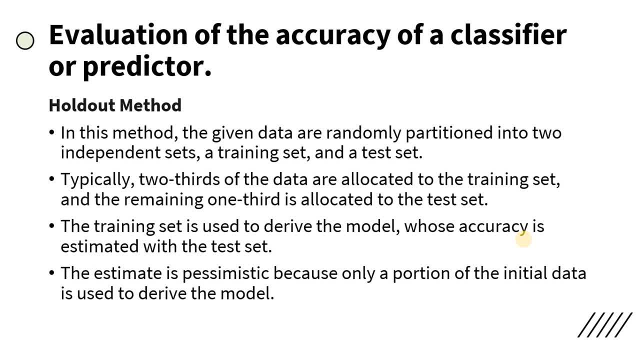 the training data set. we are taking most of the portion in the training sets and a small portion as a test set. suppose we are taking 75% of data as a training set and 25% of data in a test set. So typically two thirds of the training data set. we are taking 75% of the data as a test. 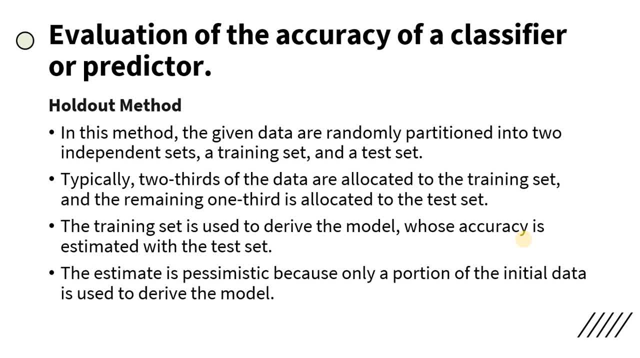 set. So two thirds of the data are allocated to the training set and the remaining one third is allocated to the test sets. So here we are using measure data in the training. the training set is used to derive the model whose accuracy is estimated with the test sets. so when, once we are building the model, 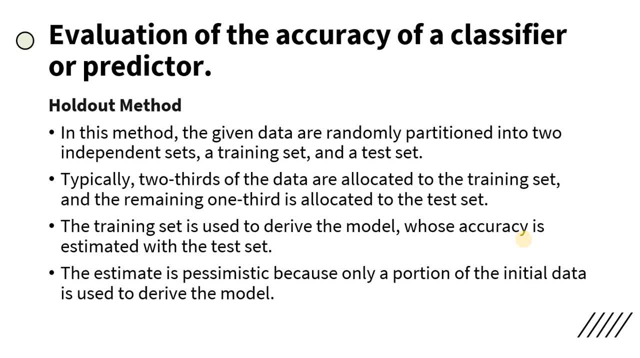 after that we need to provide training to that model so the model can learn from it. yes, So here we are using the training set and after that, to check the efficiency or to evaluate that model, we are using the test data sets. So this is a simple method. it is called the holdout method, in which we are providing two 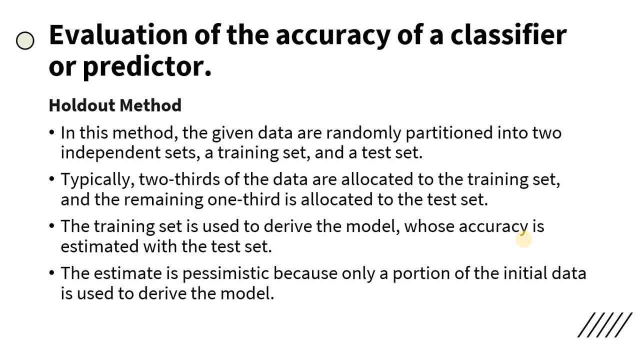 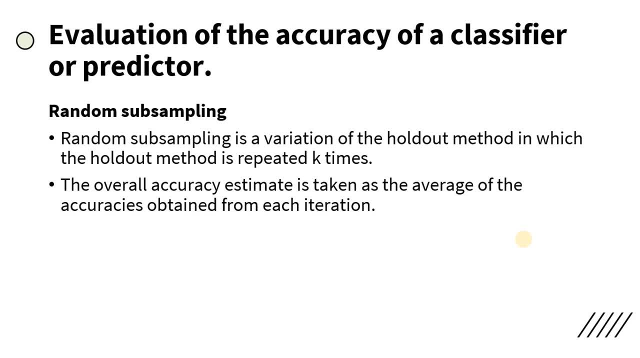 thirds of data into the training and one third into the test data sets. The second method is a random sampling, while in the random sampling, random sampling is a variation of the holdout method, In which the holdout method is repeated k times the overall accuracy estimate is taken. 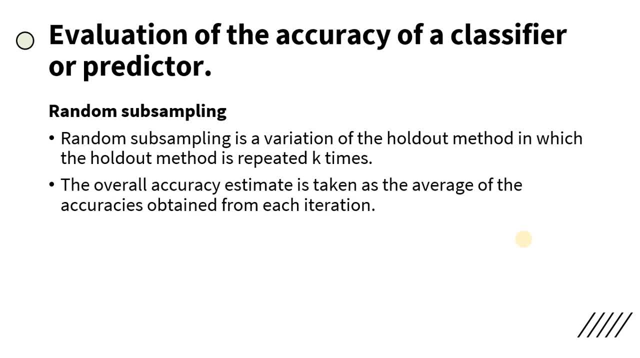 as the average of the accuracies obtained from each iteration. Suppose we are taking 75% of data in the training and 25% of data into the testing. we are repeating this process, suppose, 10 times, so result of each iteration is different. so we are taking 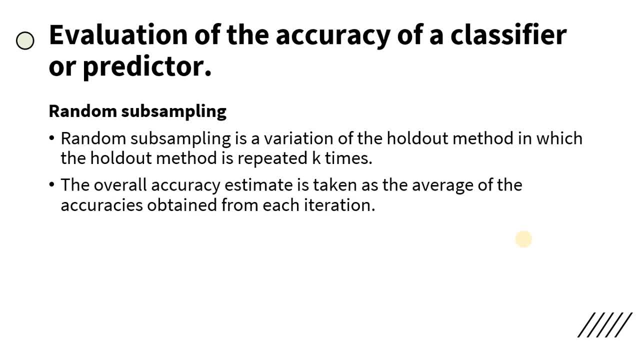 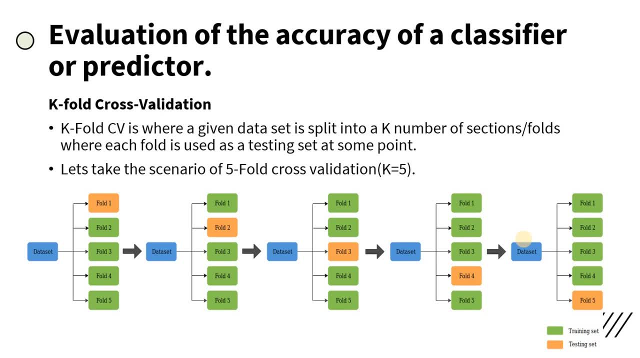 the average of it And then we will calculate the final result. so that is a random sampling. Fourth one is a k fold cross validation. it is very important method to evaluate the accuracy. yes, mostly in the classification algorithm we are using the k fold cross validation method. 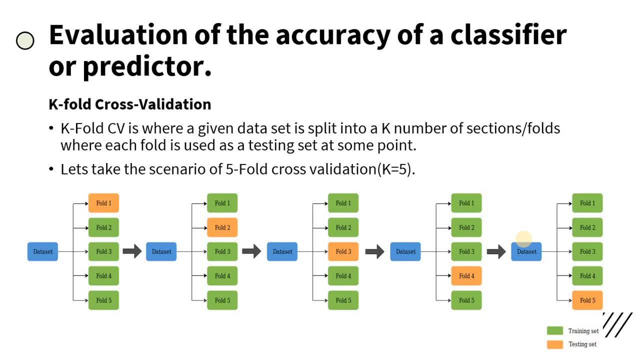 in the k fold cross validation method we are given a data set and we are splitting into the k numbers of sections. suppose here we are taking the k is equals to 5. it means the data set is splits into the 5 folds. so in the first iteration the first fold is used. 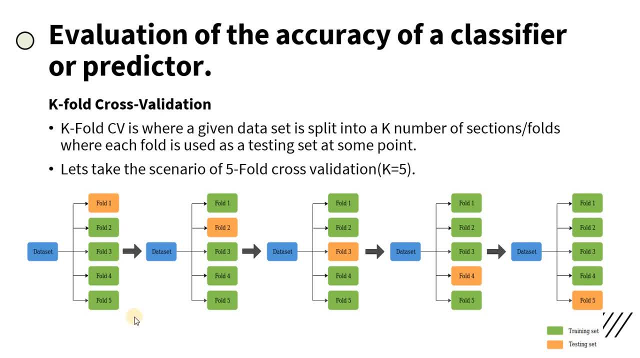 to the test model and the rest 4 are used to train the model. in the second iteration the second fold is used as a test data set and all others are used. in the training data set, same as in the third iteration, we are using fold 3 as a test data sets and all 4s. 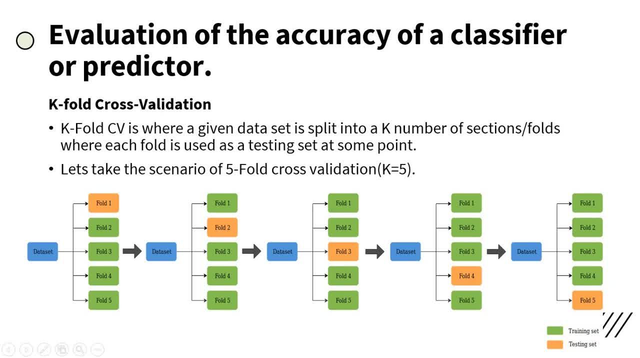 rest of the folds are in the training data sets and so on. so what is the benefit of it? we are taking a whole data sets in the training. yes, because in the fold one this whole rest of the four data set is given as a training to the model. after that this fold one is also given into the 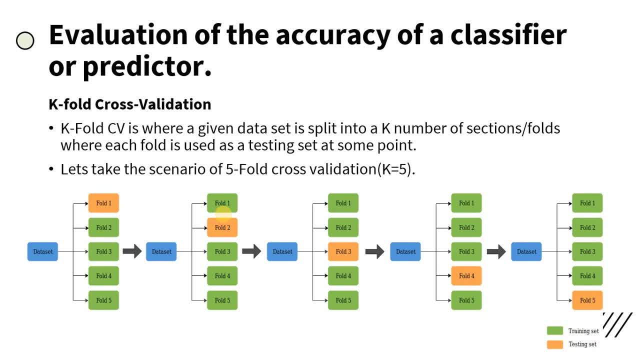 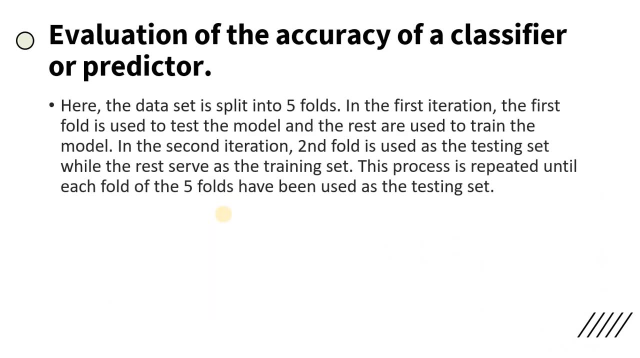 training. so each and every fold, so each and every items in the database will be used in the training. so model can easily classify the new data, yes, test data. so the accuracy of the model will be increased. and the last one is a bootstrapping, so technically speaking, the bootstrap sampling. 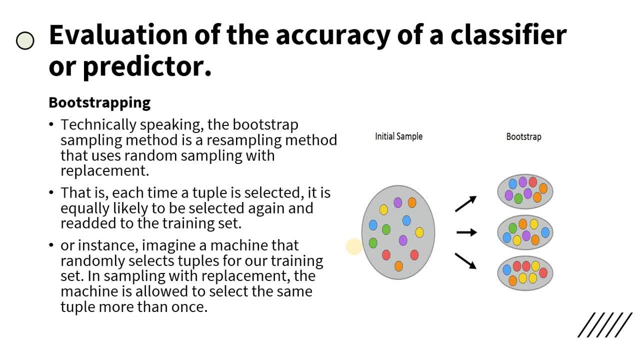 method is a resampling method that use a random sampling with replacement, that is, each time a tuple is selected and it's equally likely to be selected again, and related to the training sets. or instance imaging a machine that randomly select tuples for our training set. in sampling with replacements. the machine is 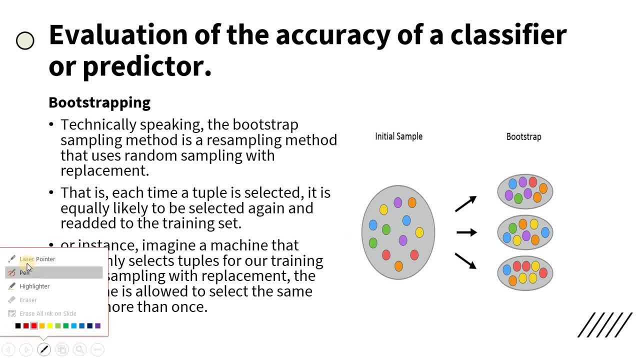 allowed to select the same tuple more than once. so here what happened? this is an initial data set. yes, now we are taking some of the data in the this first section, then others into second section, then more others in the third section, and so on. yes, suppose this is a data. 1, 2, 3. now.